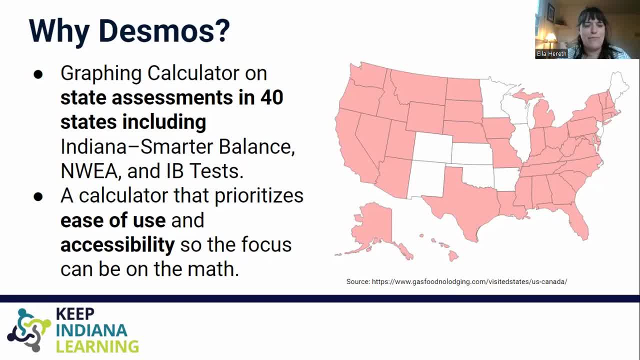 and memorizing a whole series of buttons on my TI-84 to try to remember my graphing calculator, to try to remember how to get to certain features, And Desmos really tries to not be that. So the less time we can spend in class memorizing buttons to push and the more time we have to focus on the. 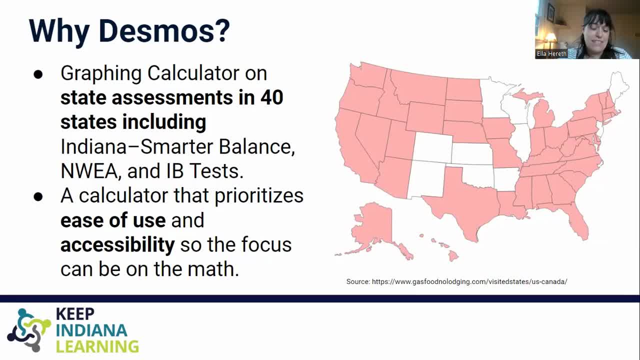 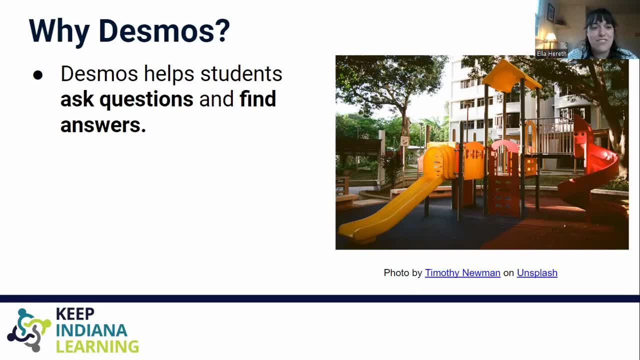 math And I will show you a little bit of that ease of use. And the other reason that we should be using Desmos is it really helps Students ask questions and find answers themselves, And isn't that really the goal of math class. We'll talk a lot about what if and just a whole series of what if questions that Desmos 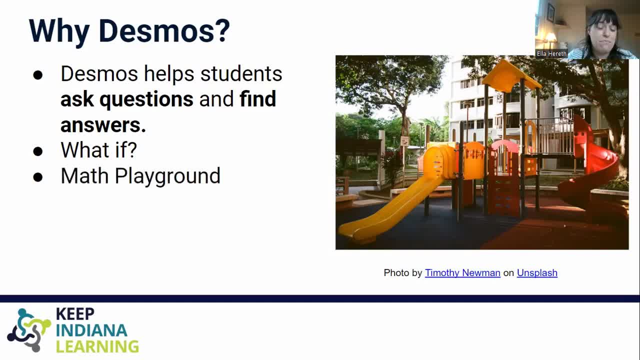 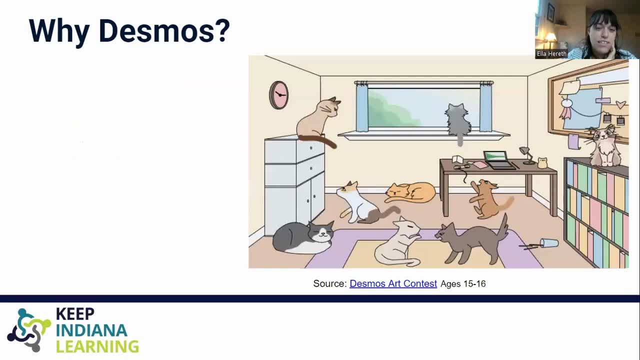 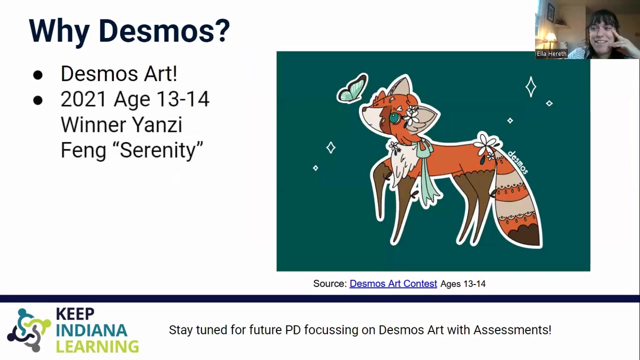 graphing calculator can spark, And then we really hope it can be a playground. One example of how it's become a playground is through the amazing Desmos Global Art Contest. This is the winner in the 13 to 14-year-old category. Again, amazing, amazing stuff. And again you can click on the link to: see the actual calculator. And then you can click on the link to see some of the animations as well too. And open the folders and look at the math. Here's the winner from the 13 to 14-year-old category. Again, amazing, amazing stuff. And again you can click on the link to see the actual calculator. 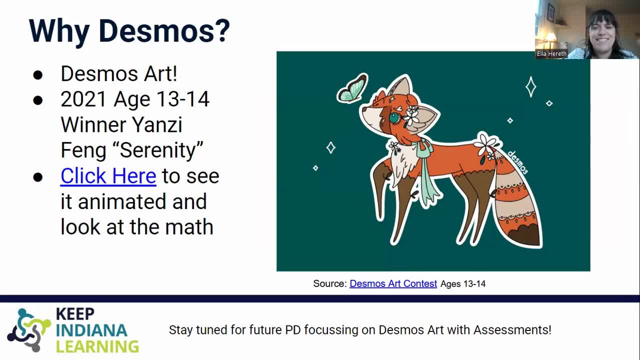 And then you can click on the link to see the actual calculator. So you'll have a calculator link and the folders. so look at the equations and see the animations, the mathematical animations in there. So stay tuned for some future PD position, future blog post. 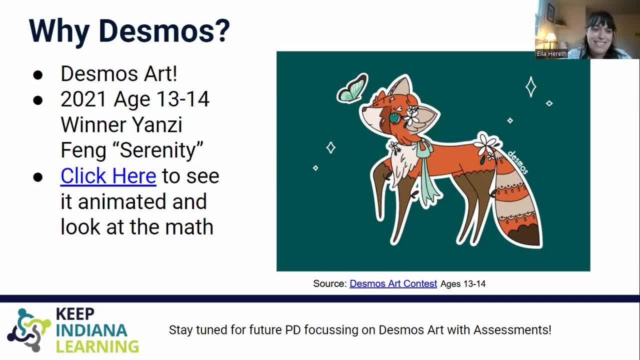 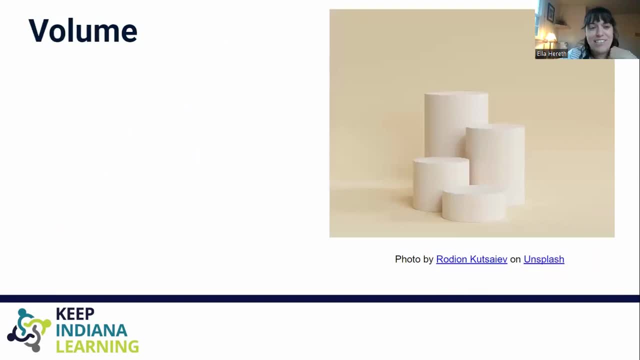 discussing Desmos art and how to assess with Desmos art and some ideas at some things that I've done in my actual middle school algebra classrooms in Indiana. So let's jump into the actual problems. so we are going to look at two problems. 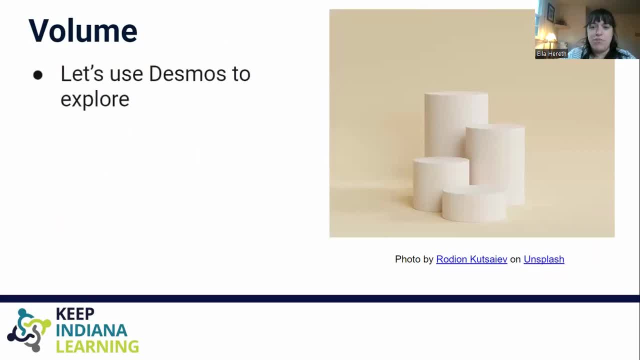 here One is just a classic exploration of the volume formula for a cylinder. You see some cylinders there in that image. So if you're like me, one of the first things I remember learning about cylinders in school was the formula, starting with the formula, And then I kind of 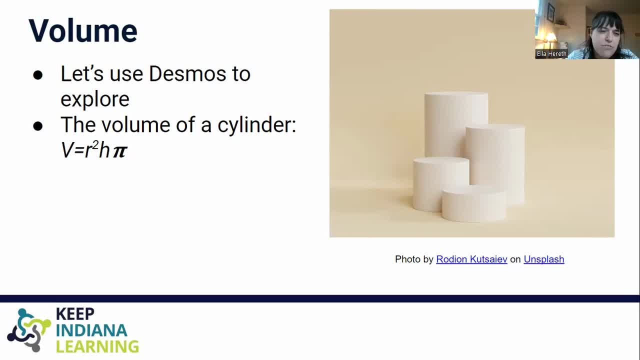 plug numbers in there and usually got the right answers. But I don't know that. I really spent a lot of time thinking deeply about that formula and what it looks like when I change different things in that formula. So I'm going to jump out of the slideshow and into a Desmos graph. 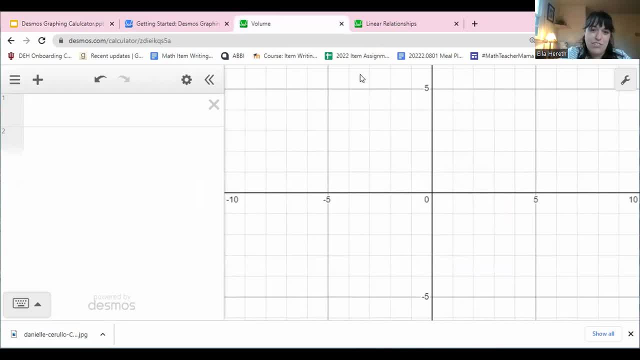 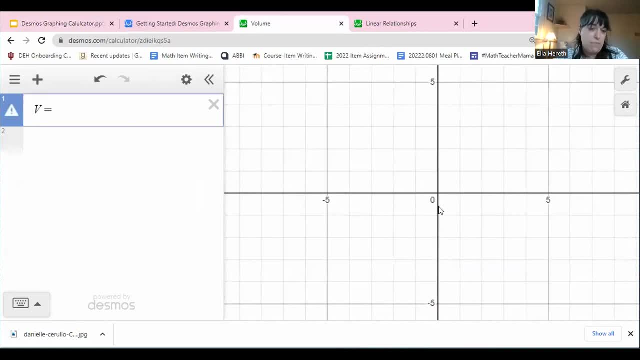 and I will link these back in the slides at the end of the presentation. So here is a blank Desmos graph And I'm going to jump in just with typing the formula. Start to get good at some of these Desmos shortcuts after you've done it for a little while. but you can also put some links at: 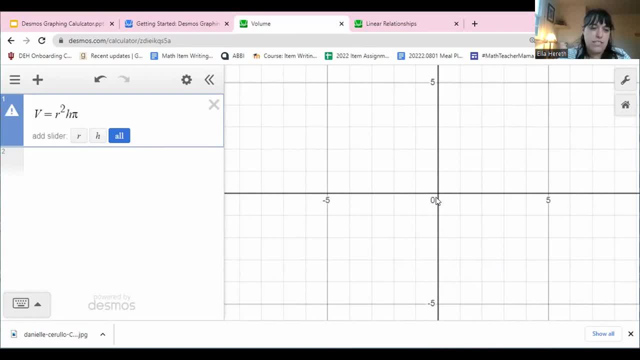 the end, so you can learn about all of the resources, But learn how to graph on the Desmos calculator And I'm going to add some sliders. So give me that little pop-up, add some sliders. I added one for radius and for height And right now the slider is: 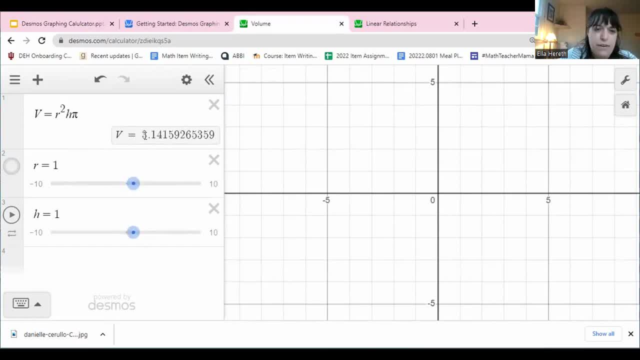 set at one. You can see that if my radius was one and my height was one, my volume would be pi, which makes sense. What I want to do is I'm going to adjust these sliders just a little bit, So I'm going to click on edit So I can see some of the things I can edit here And I am going to make. 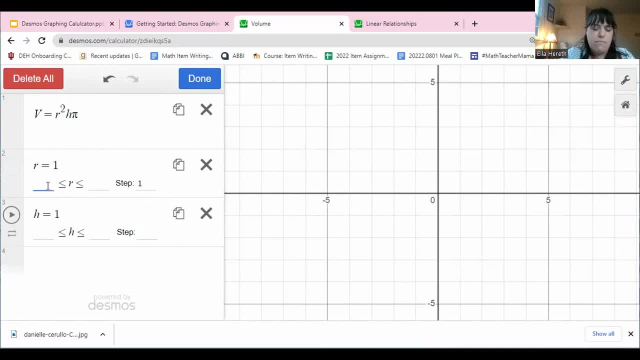 the sliders move in whole numbers. I'm also just going to make them start at zero, because I don't actually need negative numbers for my formula. So I just made them from zero to 10, but you can change the range of the slider using this: 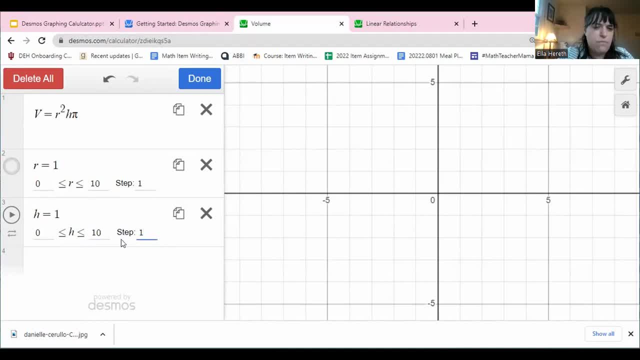 part of the graph right here And I'm going to make this one whole numbers as well. The step means what is the space of the step. Okay, So right now. now you can see when I drag the slider it can only land on whole numbers, So I'm restricted to these whole numbers. 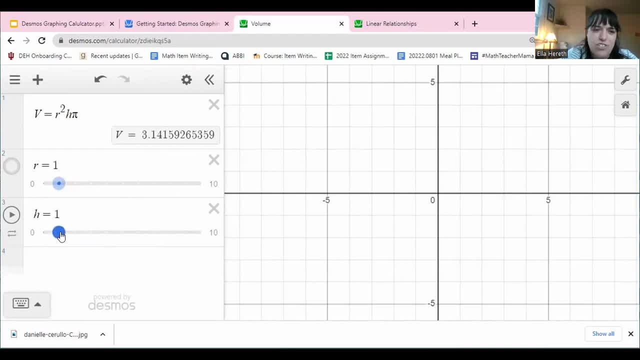 Right here let's take a look at what happens when I change height. This my answer: when volume is one and radius is one, we're going to leave radius as one in advanced height to two, And I might ask students what happened to the volume? 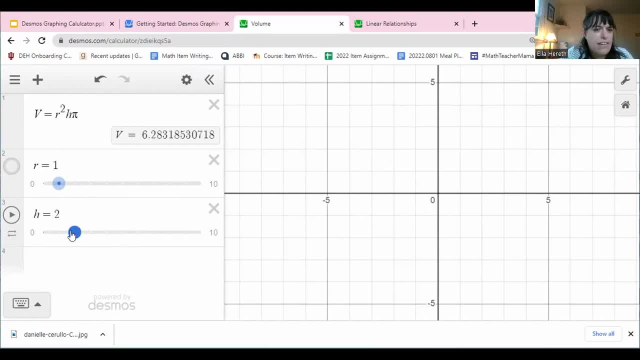 Oh, it's bigger. What's get bigger by? What are we multiplying by? And I might go back to the volume at one so they can take a look at that, Hopefully. I notice I'm multiplying by two, Okay, And notice when I changed it should be three. 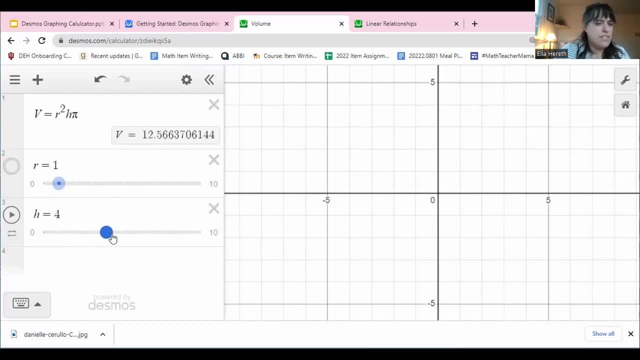 Oh, I noticed that I'm by three. Okay, great, We noticed that when we change the height, we're basically changing the volume by that number, by scale of that number. Yeah, Okay, Let's take a look at what happens. 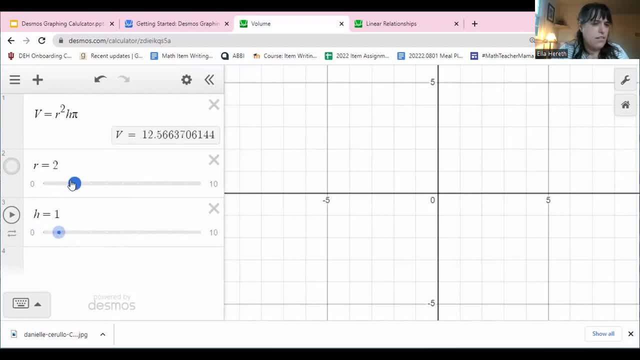 when we change radius. Okay, Here it is when it's one, Here's when it's two. What did you notice? Oh, Ms Harris, that changed that more than changing the height. Yeah, I wonder why, And students might also wonder why, And then they might find that answer in the equation: It's. 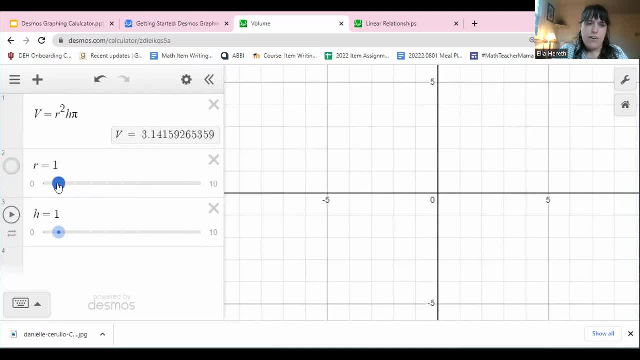 because it's squared in the equation. Oh, what are we multiplying the volume by when we change the radius to two? Oh, we're actually multiplying it by four. Changing the radius to the two is the same as the volume we get when we change the height to four. I wonder why Students might. 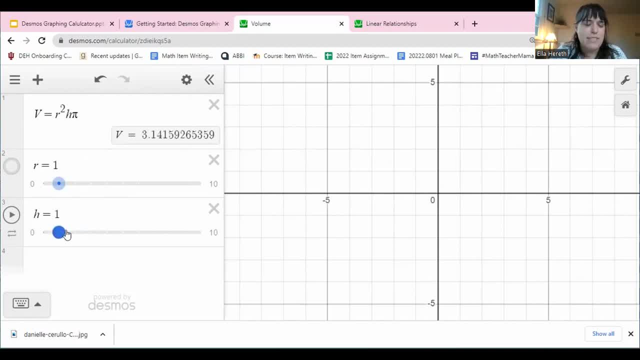 come up with that answer? Oh, it's because it's two squared. So there's rich exploration that I can get just by looking at the formula in the graphing calculator and moving some sliders around and having a conversation. You can do that with any formula that you're learning about as you're exploring volume and 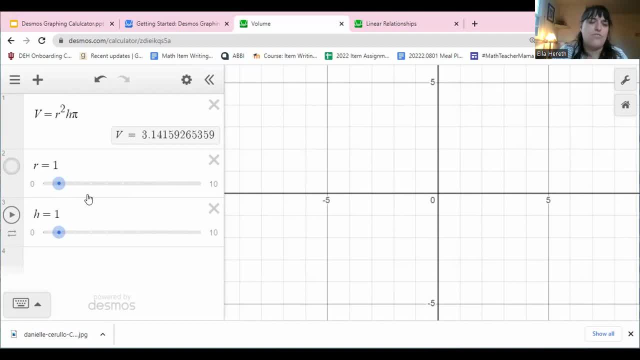 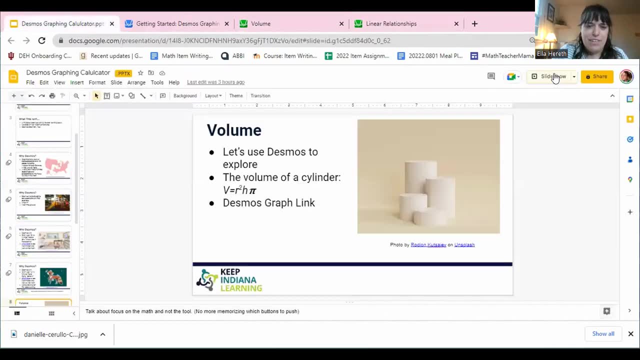 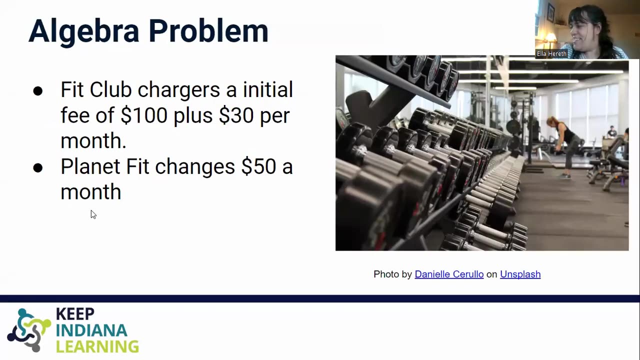 surface area And it really connects the radius and the height to that equation. Okay, So that was our first problem I wanted to briefly explore- And I'll put a link in there- And the second one we're going to explore. I'll also add the link here at the end. The second: 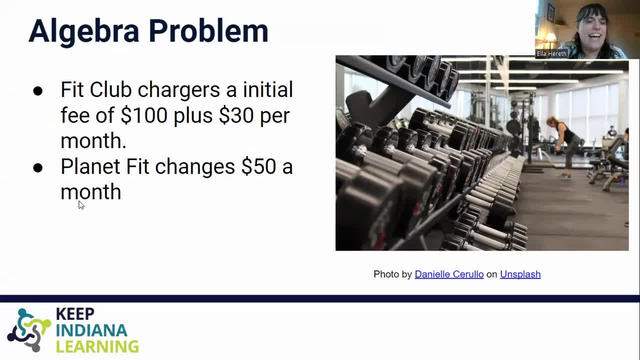 one we're going to explore is this algebra problem. So this is a classic algebra problem. We're going to do it in a little bit, And then we're going to do it in a little bit, And then we're going to trend. So I'm going to jump the new bar up to the first point again, And 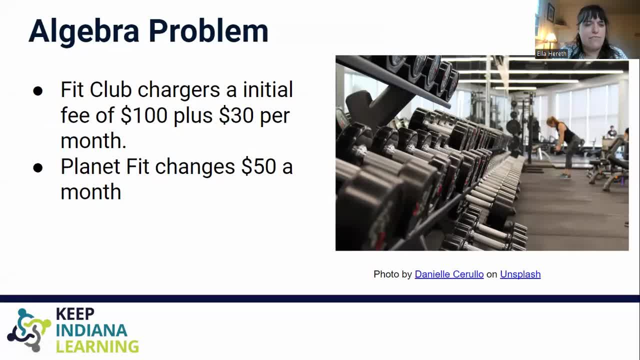 what I was thinking of in this picture is some real- world stuff here I'm here. You can see just who makes the difference between墨 andพ And, honestly, Africa's pretty popular here. So what made all this difference? you can see Los Angeles, Texas. they have a Path College. 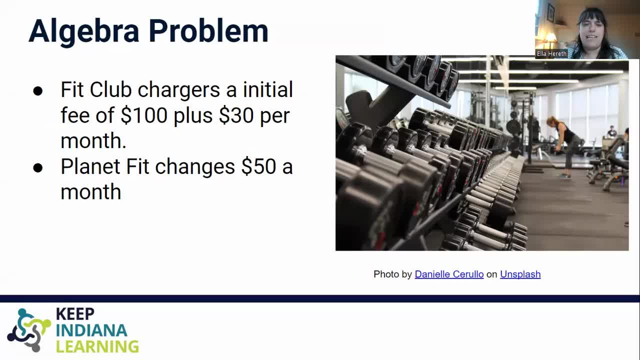 that sells foarte well. but 두�יםون marque and gems Los Angeles' was that it's still looking up in June. So you'd think it was going to be a conflict or it was going to be detectable. But when you do the math you're seeing all. the different objects in one area. they just all come together, which is really delicious. So that's what I wanted to explore. first, A break listening to the numbers. want to show Comb shadows, or you can be one way to explain that, Because, again, if you have one group, 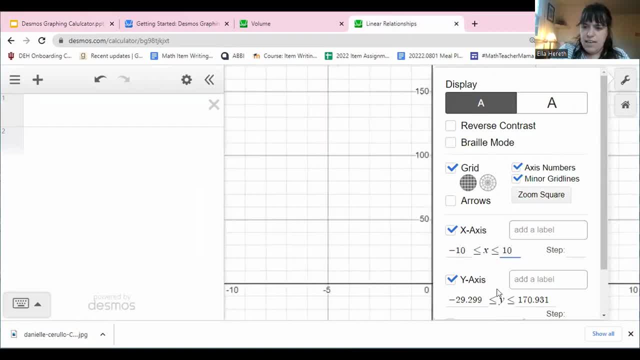 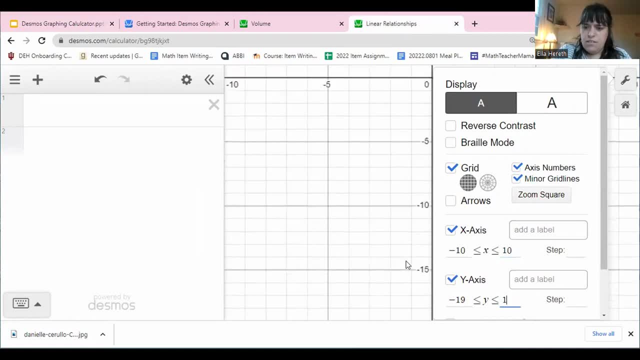 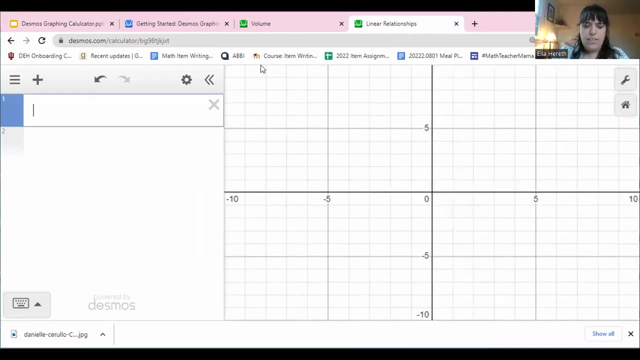 just 10 and 10, so I can show you kind of what happens if I started from the beginning: 10 and 10.. Okay, This is what we might get if we just opened a blank graphing calculator, And one of the things I love is that I don't need to use Y. We have context in this problem. It's not a. real thing. So why not use F, Because that's my club, That's the name of Fit Club. It's $30 a month And then initial fee of $100.. Okay, That one was Planet Fit And that one was $50 a month. 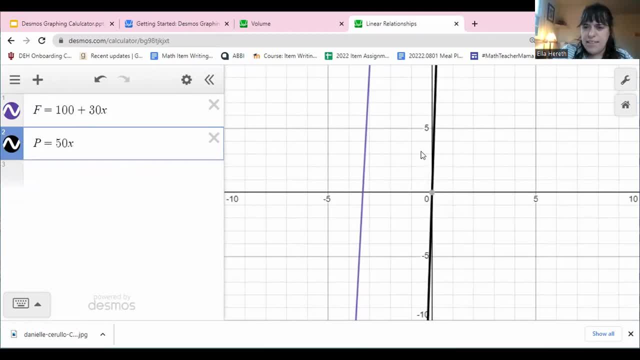 50X. Okay, So now I got my colors here. It can help me think about these. I can change the colors if I want one to be blue and one to be purple, One to be blue and one to be different colors And blue, red. Let's do blue and red, Okay? And 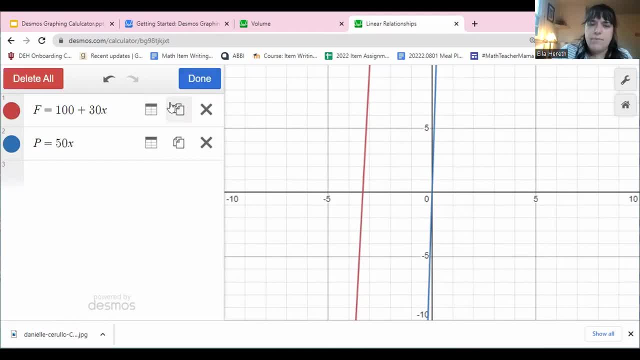 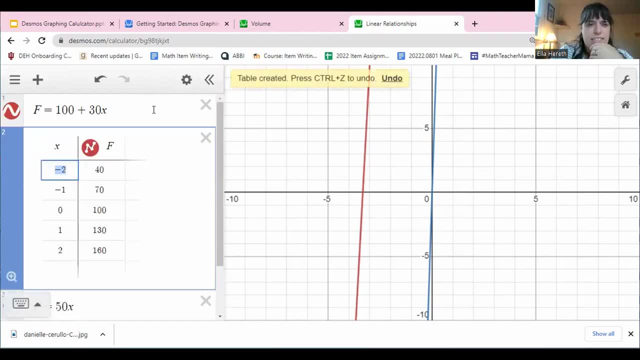 then here's some other things I can do. So this little gear allows me to do a bunch of things on the side here. So let's say I want to see this in a table. What does this expression look like in a table? I can just click on that table link and it's going to create a table for me. It starts: 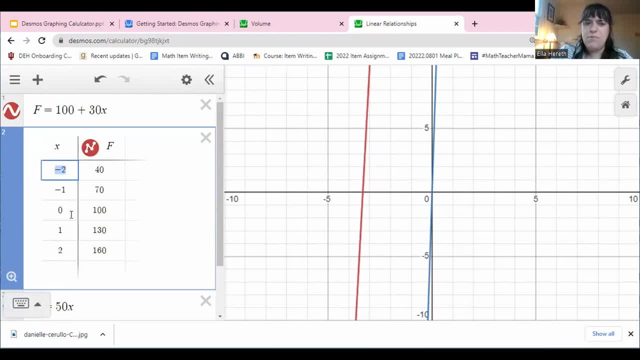 with these values. But I can really see, okay, at zero months it's going to cost $100.. At one it's $130.. And then I'm going to click on this little Zoom Fit link right here on the left And what it's going to do. 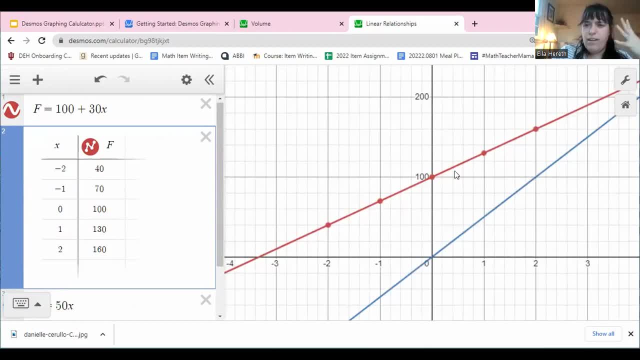 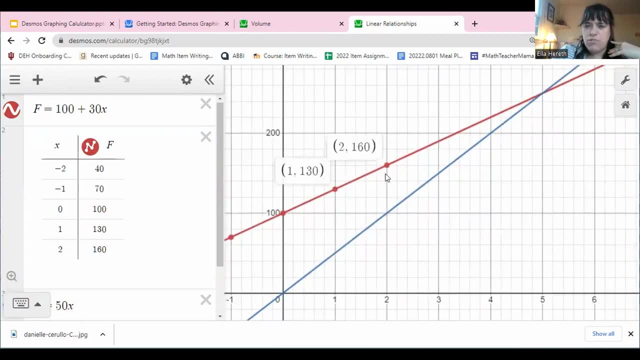 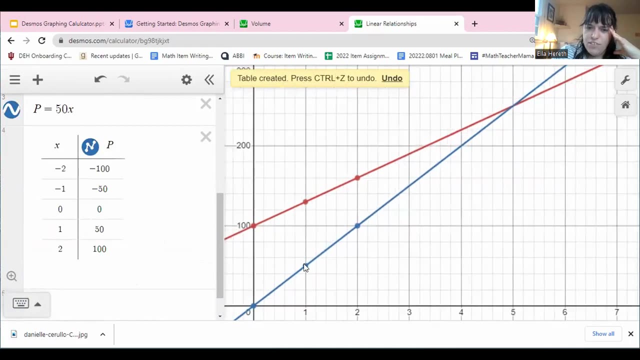 is automatically zoom that graph into a great fit for that graph. So now I can see some of these values on this table And I can really just explore. to just look at Quadrant 1.. That's the one that makes sense here. That's a table for my second function, And then I might ask students. 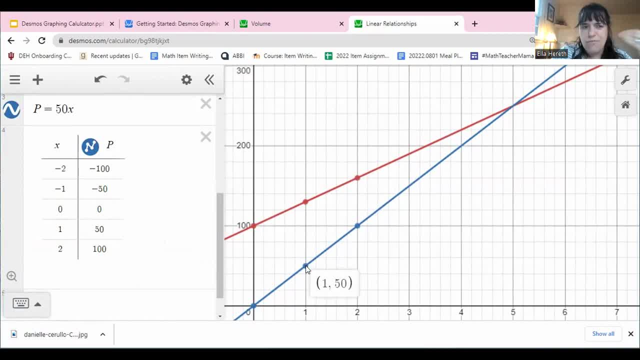 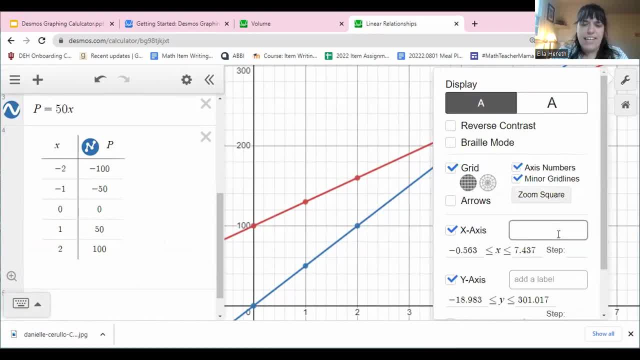 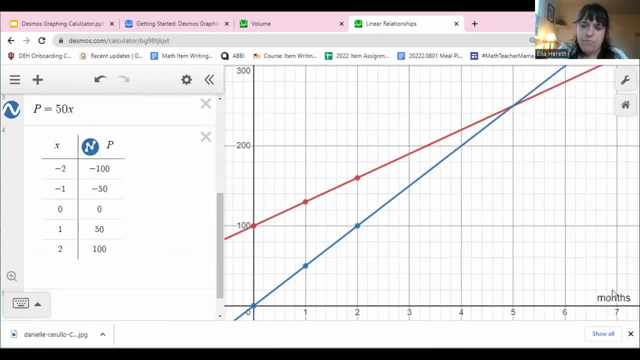 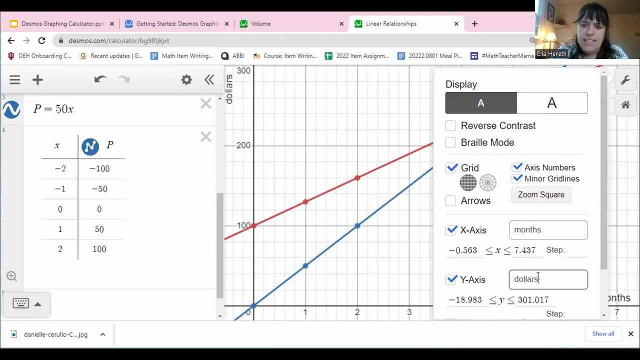 Let's add the word months to the X axis And you can see. it shows up right down here. And what did you tell me? the 50 and the 100 was? Oh, that was the dollars that you pay. So let's add the $100. 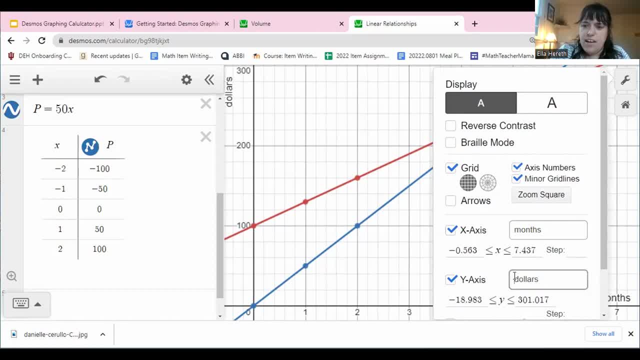 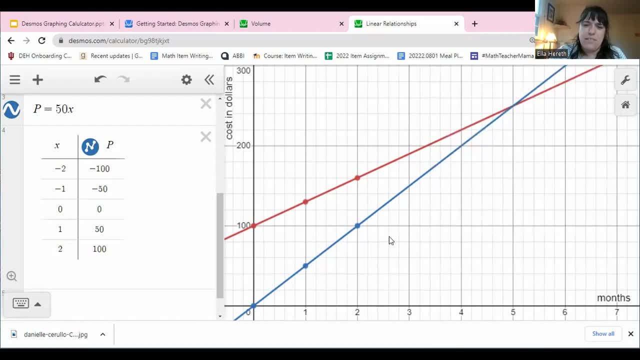 The word dollars to the or the cost in dollars to the Y axis, Because that's what we're talking about on the Y axis. So we're making sense of some of these numbers and some of these numbers in the table. Then I might ask students: okay, how many months do you think it would be until? 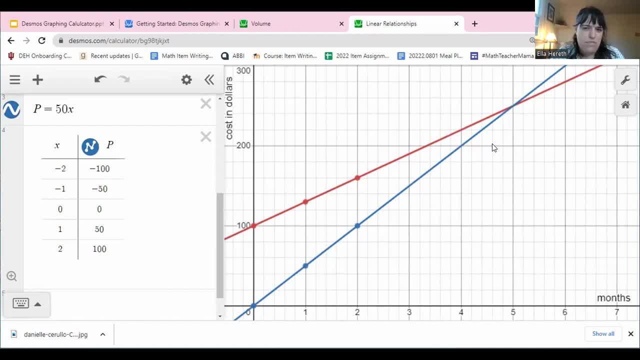 you paid exactly the same amount at both of these places, And hopefully some students might come up with an answer. Ms Harris, I think it's five. Why do you think it's five? Well, if you see the answer it's five. Why do you think it's five? Well, if you see the answer, it's five, Well, if. 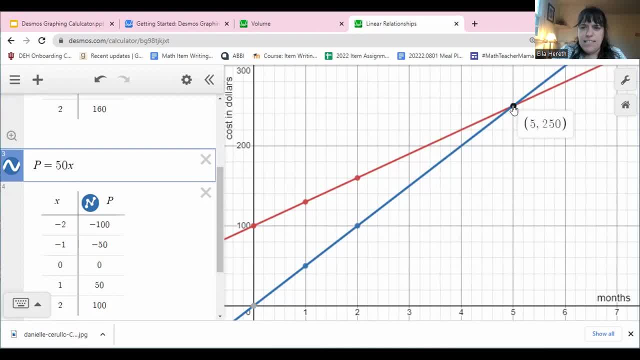 that's where the lines cross. if you click five, you can see that at that point it's on both of the lines And I might say: okay, well, what do you think they would pay at both gyms after five months? And they might say $250.. How did you know that? Oh, it's from that point, right there. So 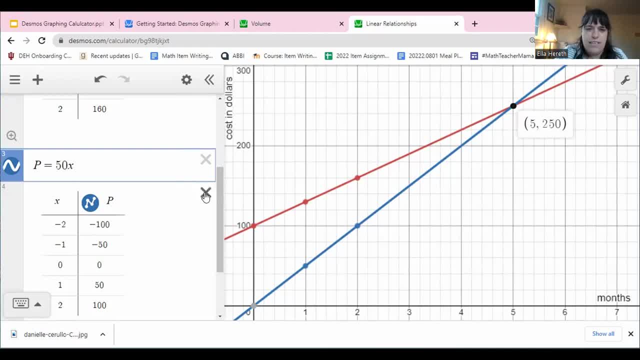 much rich exploration, And you can do even more with this, So I'm going to delete some of these tables. give us a little more space over here so we can see, And let's turn these into functions with F of X, Ms Harris. 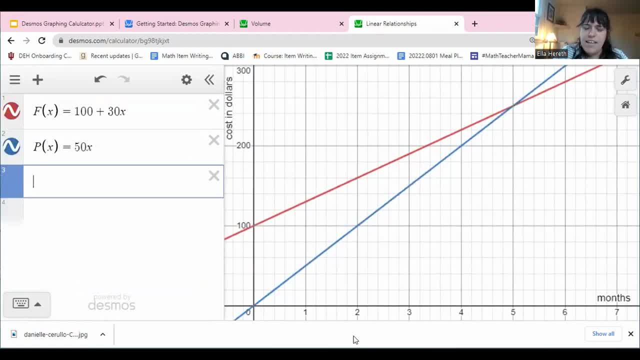 Now I'm going to add another one. So what would happen if I did S of X and it's going to be the cost at one gym minus the cost of another. Oh, that's how much I'm saving if I'm going from this. 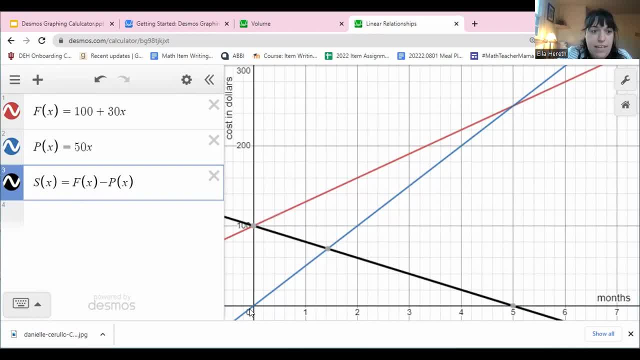 gym, or the S of X, F of X, the planet. this one minus this one, So I'm going to add another one right here. Amazing. So zero months. I'm not saving anything. I'm spending a hundred dollars more. What do you guys notice about this graph? Oh, I noticed that at five it's zero. So after 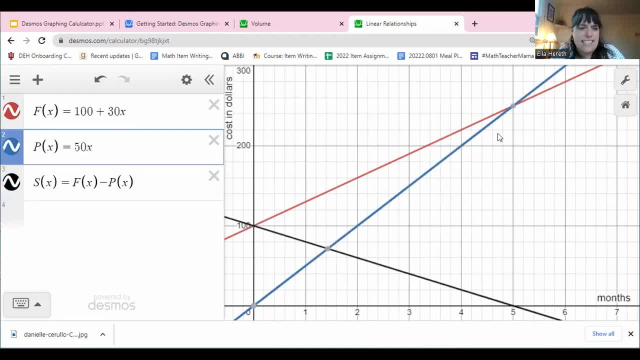 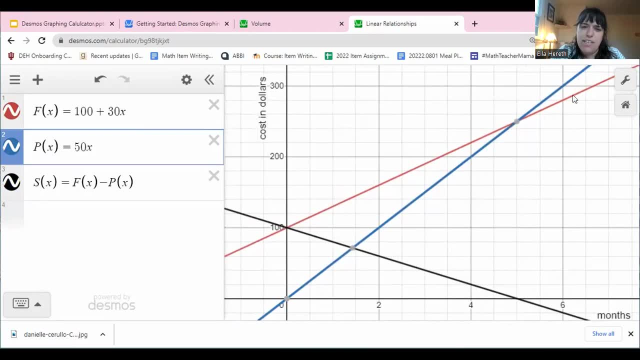 five months, the cost is going to be exactly the same. And then what about the other ones? Okay, Well, now it's going to be negative, because you're no longer saving money by going to this one, because now this gym is going to be negative. So I'm going to add another one. So I'm going to 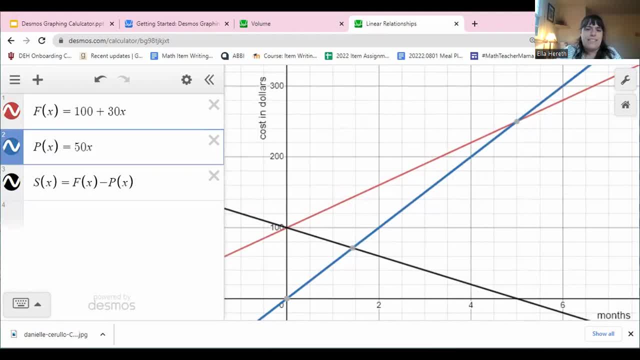 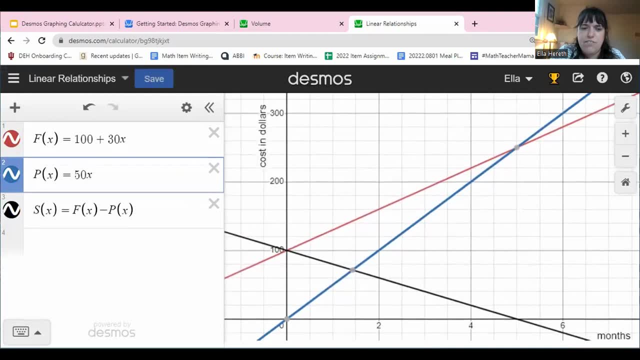 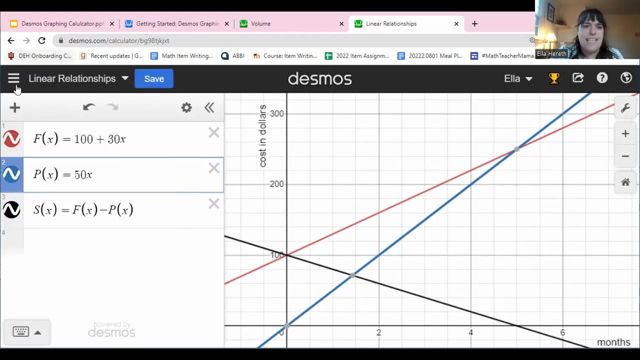 cost more than this gym. So there's so much rich math discussion that you can get by putting things into this graphing calculator and exploring it and talking about it. So I just really encourage people to kind of just explore and play around. I am going to link to that these two graphs in: 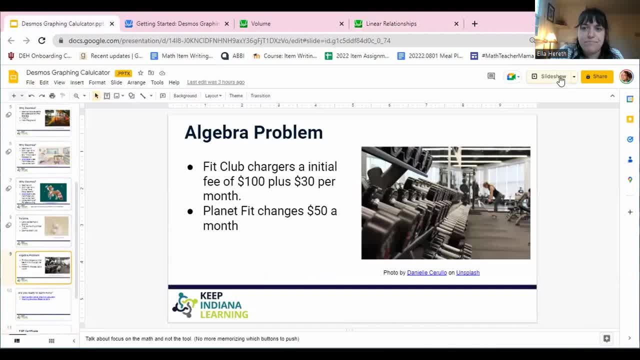 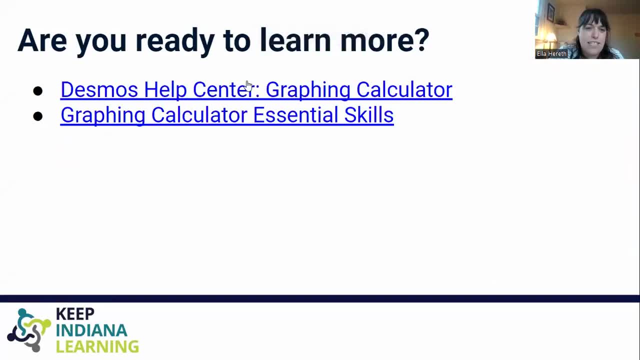 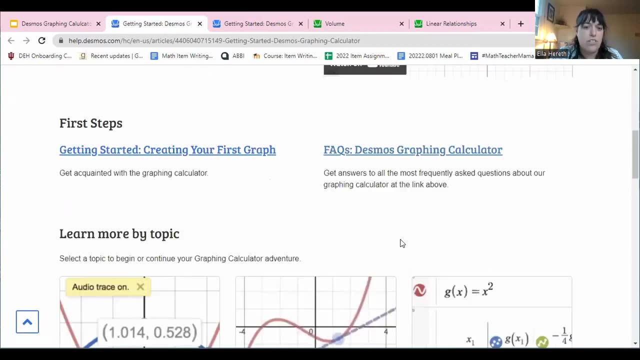 the slideshow that I'm sharing as well. And then my last few things. to really think about it are these two links right here. So if you are interested in learning more about this, you can go to this link, the Desmos Help Center. There is just such a huge set of resources on how. 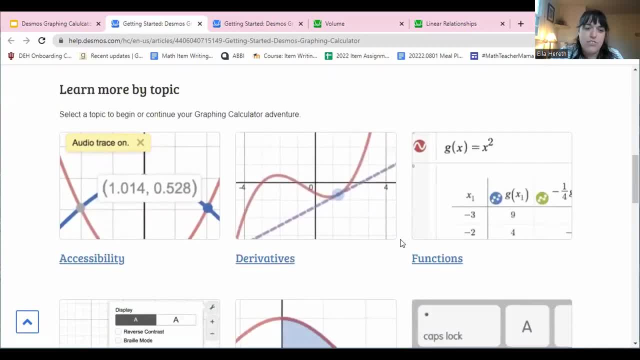 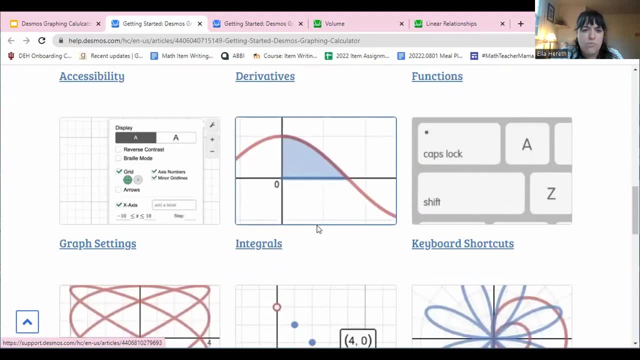 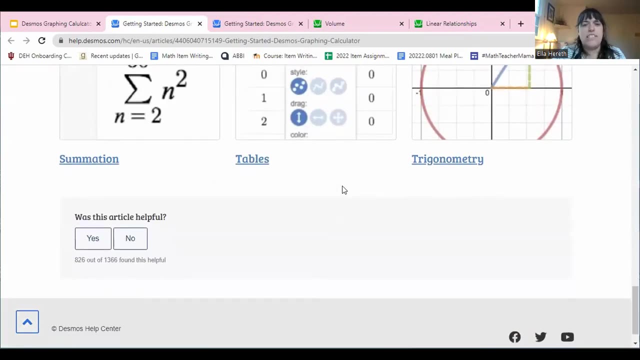 to graph things- So frequently asked questions. but also, you know anything you might need to graph. What if I'm working on functions? What if I'm working on derivatives, integrals, parametric equations, polar graphing, sliders, statistics, like just all these amazing things? 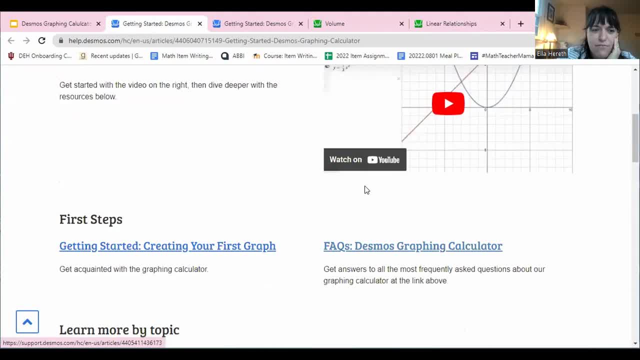 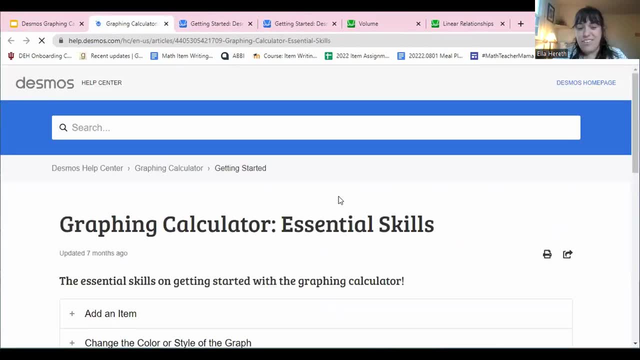 that you can do in the Desmos graphing calculator. So definitely check that out, This link out, And then the other one is: as you're building, you know kind of your essential skills on a graph. consider going through these little links to think about: okay, how can I change? 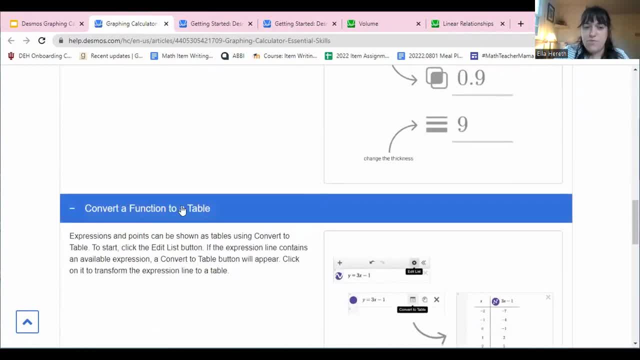 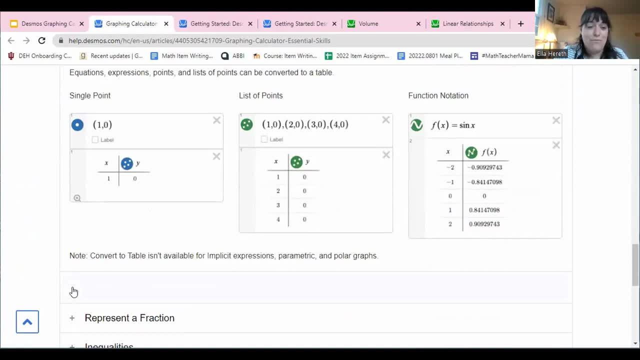 the color. How can I convert a function to a table? We did that in this animation or in this PD. How can I add domain and range restrictions? So all these little things that you might want to adjust you can find in kind of this link out. And then the other one is: you know, 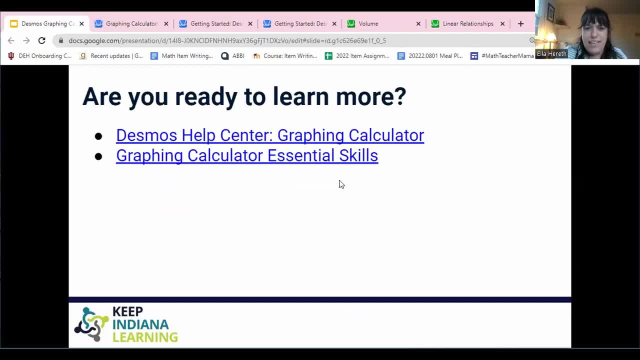 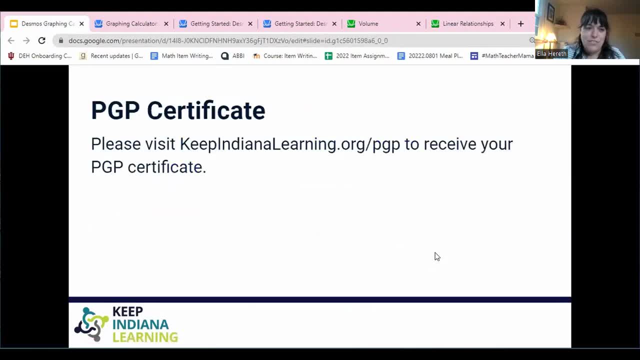 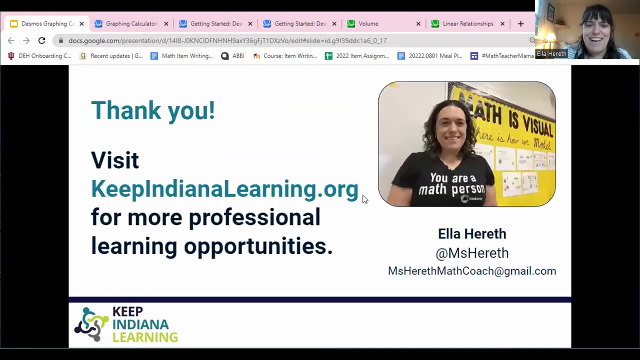 the link out. Thank you so much for coming and learning just a little bit about it from me, And I really hope that you will consider doing some content exploration with Desmos graphing calculator and that you will continue to work towards- you know- developing a deeper understanding of the math using this calculator in your classroom. Thank you so much for coming and learning just a little bit about it from me and my students. Thank you so much for joining me today And I look forward to seeing you next time. Bye-bye. 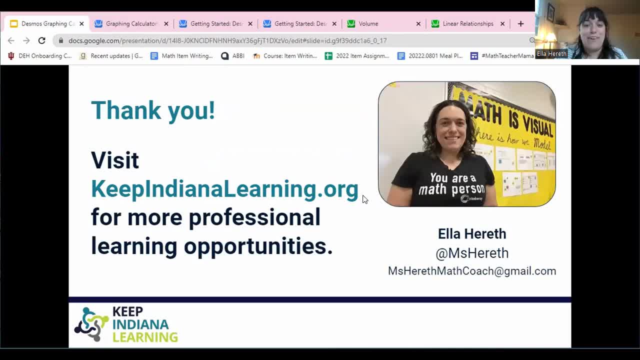 me right now, And I'd also just really encourage you to reach out with questions. I always tell people that my number one goal is that Indiana can be the center of math exploration and math learning, So I really just want to make that happen. So please reach out to me, talk to me. 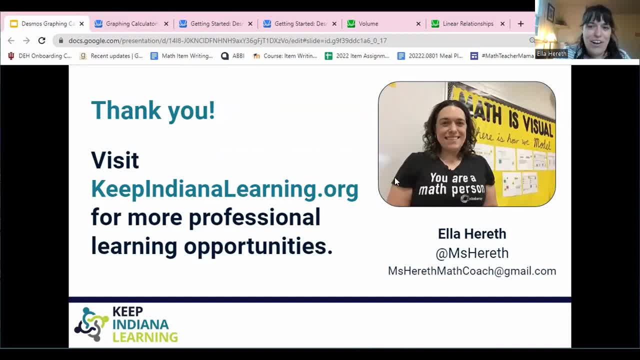 about Desmos and or all the other amazing things going on in Indiana math classrooms. Thank you so much.